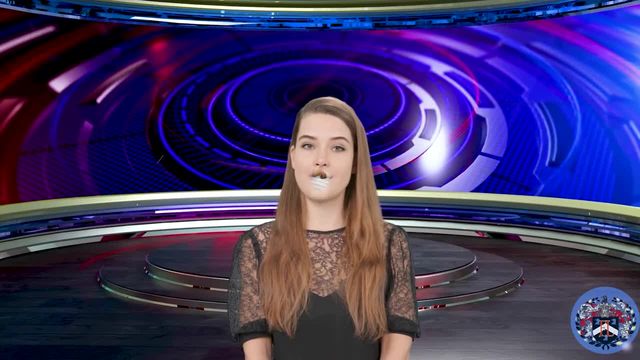 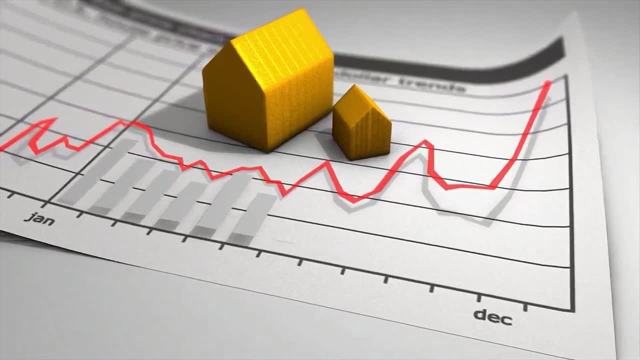 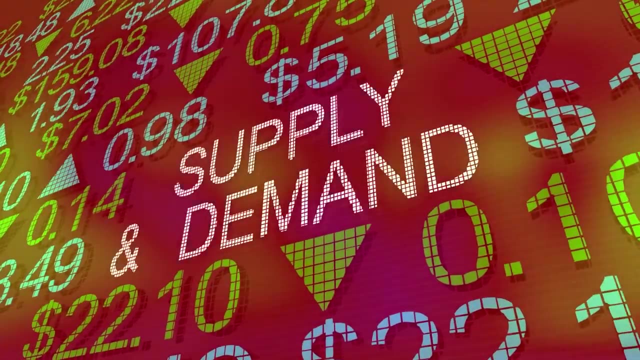 which similarly eroded real income and economic stability. Currently, individuals who secured mortgages at historically low rates are reaping substantial benefits from inflation, which effectively reduces the real cost of their investments. On the flip side, construction companies face mounting pressures from rising labor and material costs. This surge widens the gap between the actual cost of labor and material costs. This surge widens the gap between the actual cost of labor and material costs. This surge widens the gap between the actual cost of labor and material costs. This surgeahahshair mammICK. 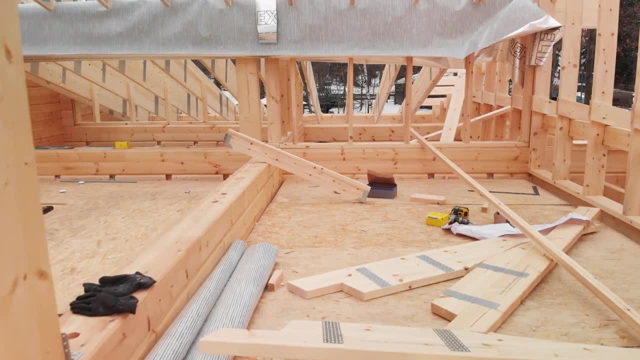 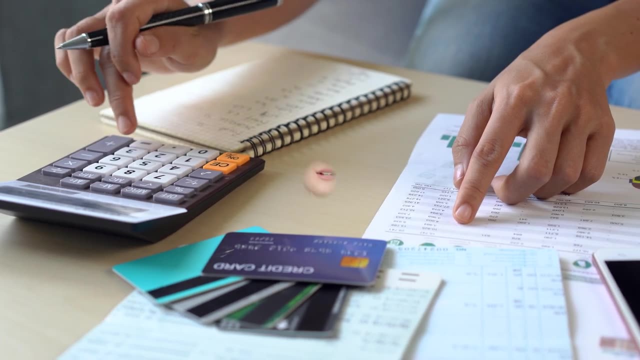 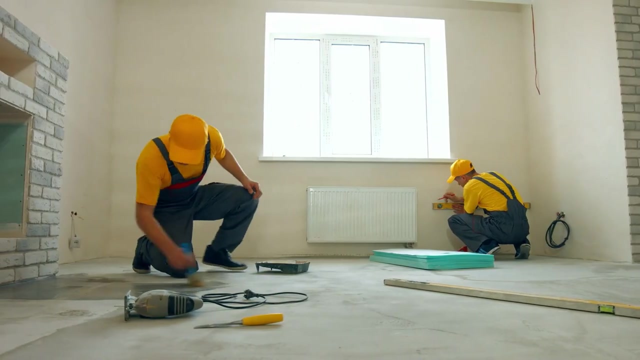 ofs and what the market can bear, skewing prices unfavorably against the middle class. This situation represents a significant and troubling financial exploitation of the middle class, unlike anything seen in recent times. Nevertheless, there are still opportunities amidst the turmoil: existing properties requiring renovation, particularly from sellers willing. 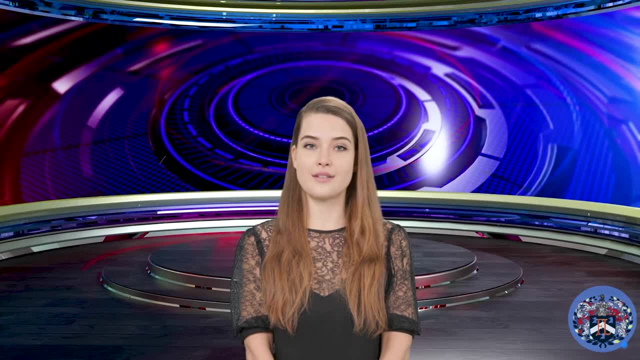 To subordinate equity present viable investment prospects. This approach focuses on generating wealth through production, aiming to transform the current debacle into a historical footnote, Instead of despairing over the conflict between short-term income and 고 ваш network's life and developments in any field. launchfan of gold and made a short-term genres which 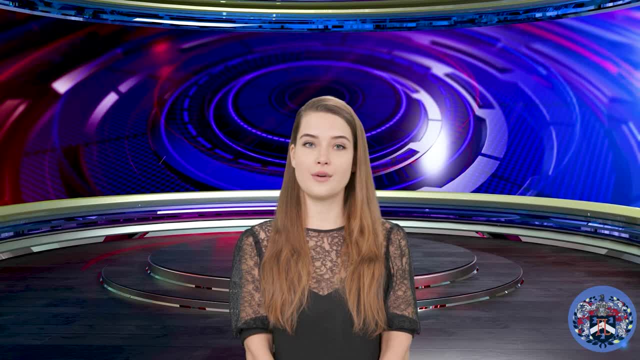 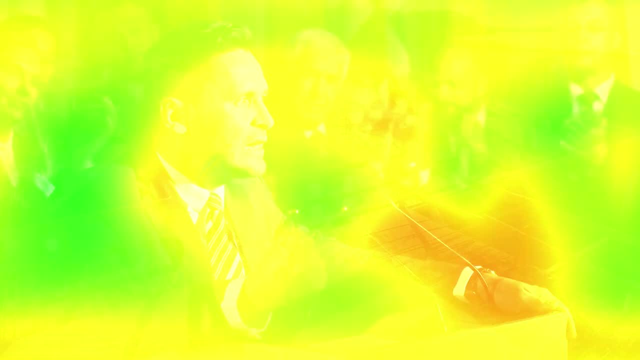 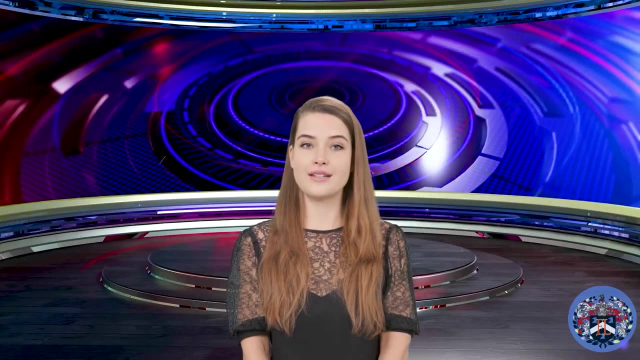 bearing over the current state. we should critique the misguided notions of so-called economic experts and face the absurdity of our situation with a resolve to find practical solutions. In the chaos there is potential for those ready to pursue ventures that offer substantial real value beyond mere numerical inflation. Historically, our economic crisis 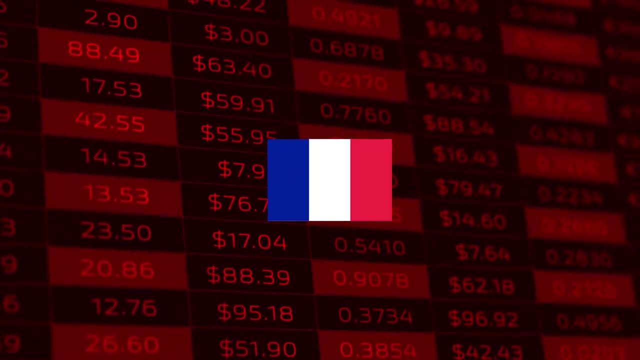 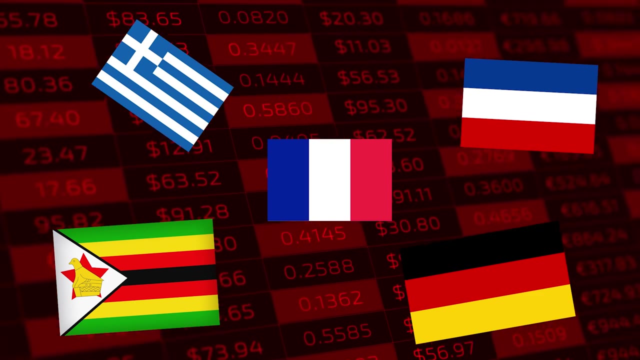 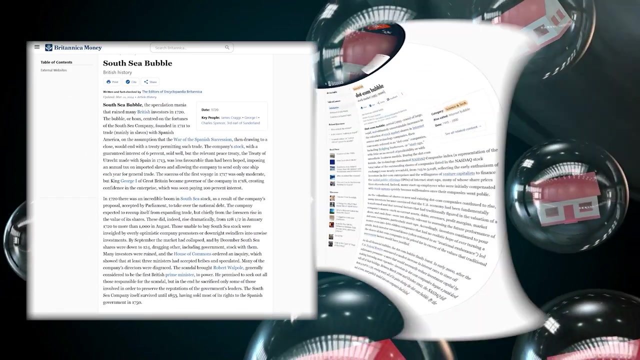 is not unprecedented. Hyperinflation in countries like France, Germany, Greece, Yugoslavia and Zimbabwe all stem from unchecked monetary expansion and poor economic governance, leading to devastating socioeconomic impacts. The current housing market instability echoes speculative bubbles like the South Sea bubble or the dot-com bubble, where initial exuberance was. ultimately met with economic collapse due to a disconnect between speculation and intrinsic value. The current scenario, with its similarities to the Great Depression's policy-induced exacerbations, underscores the need for a fundamental shift in economic strategy. Sustainable growth and prosperity depend on principles of sound economic management rooted in historical insights. 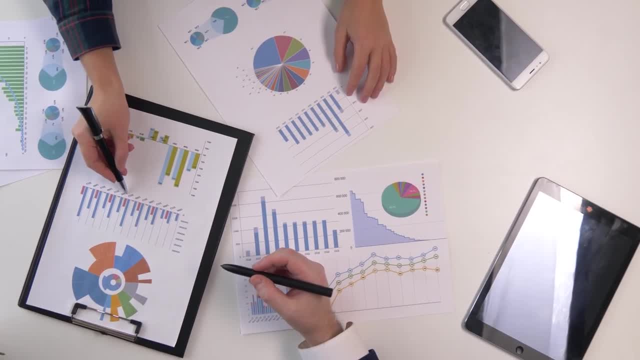 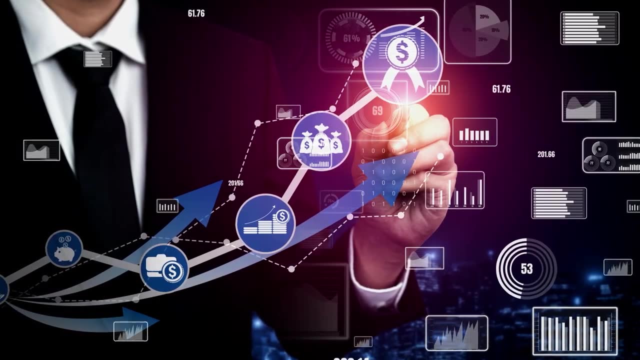 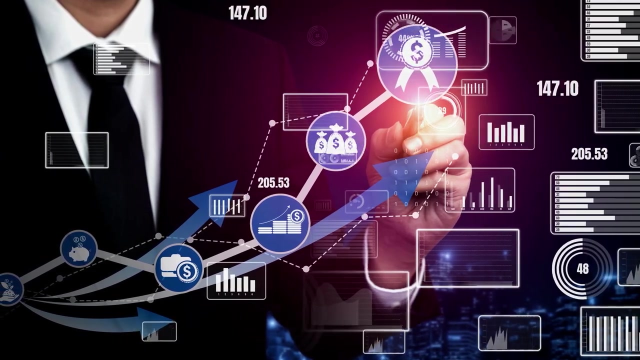 Emphasizing production and real value creation over financial engineering can guide us out of this quagmire. Adopting a philosophy that prioritizes wealth through productive endeavors rather than through speculative financial maneuvers aligns with historical lessons and provides a roadmap for genuine economic stability and prosperity By anchoring our 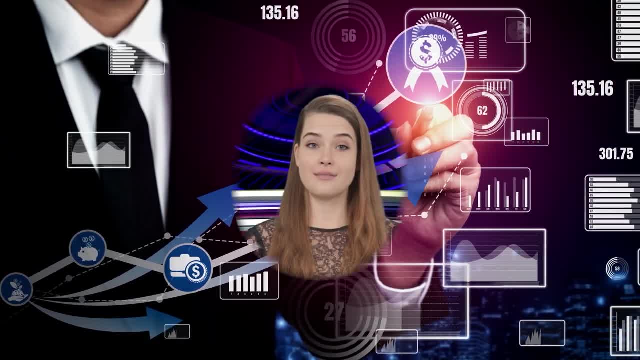 strategies. in the wisdom of the past, we can avoid repeating these mistakes and pave the way toward a future marked by genuine economic growth and stability.